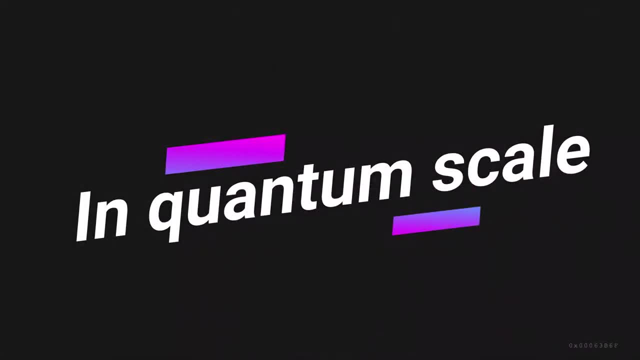 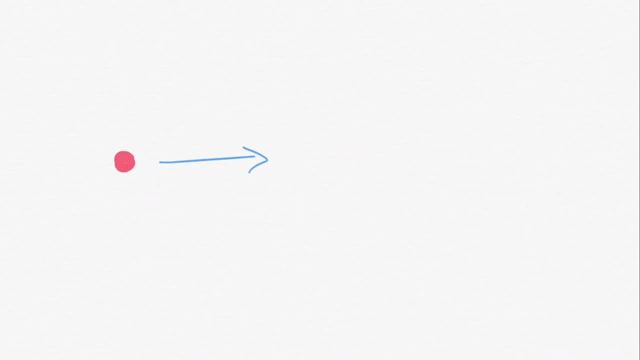 its energy. now take the same type of example at quantum scale. consider an electron which can only move along one axis, like we have taken in our previous video on Schrodinger equation, and assume that there is a barrier in the path of electron, let's say due to the electrostatic potential of an 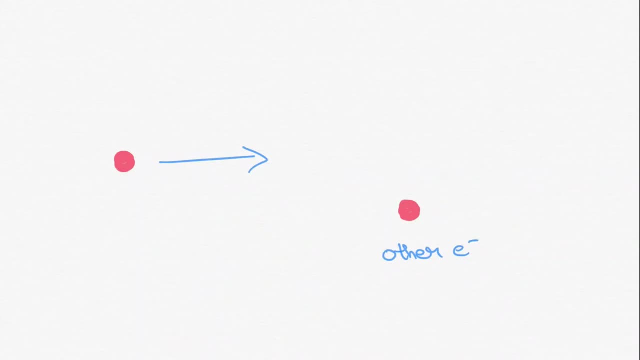 another electron. so, due to this electrostatic repulsion of the other electron, there is a region of space where the influence is felt by first electron while passing it. when first electron try to cross this region, the second electron exert force on it and if energy of the electron is not sufficient. 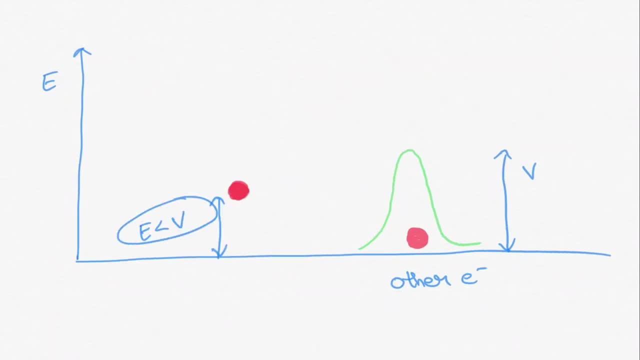 that is, energy is less than V naught, it will bounce back and remains on the left hand side of the barrier. and when energy of the electron is sufficient- larger that is, E greater than V- it can be anywhere. and while crossing the potential barrier, the speed of the electron decreases due to the loss of 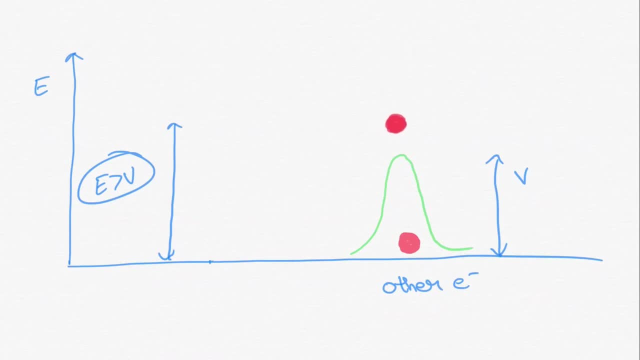 energy. so this is all classical, no excited thing till now. but when electron have less energy than the potential barrier, V naught, even then it has chances of crossing the barrier. so here comes the interesting thing, which can be explained quantum mechanically: simplify our potential barrier. just for the sake of explanation, consider it of. 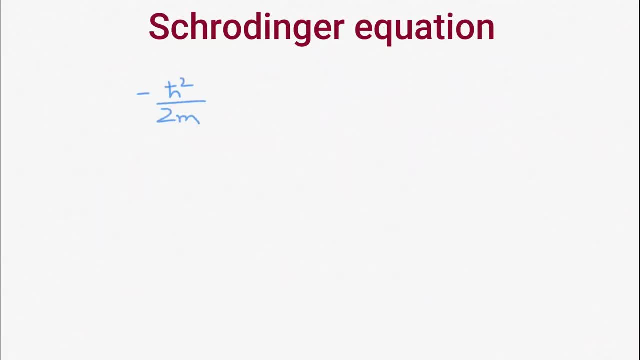 rectangular form. now we will use Schrodinger equation to analyze the problem. we have two cases: energy greater than V naught and second, energy less than V naught. case one, when energy is greater than V naught. it is not interesting as it is all classical and solution to this case is like this: and: 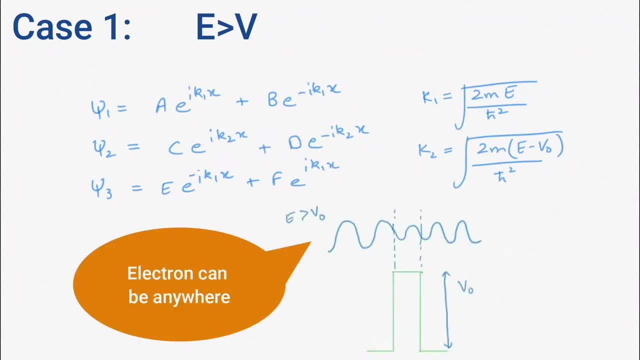 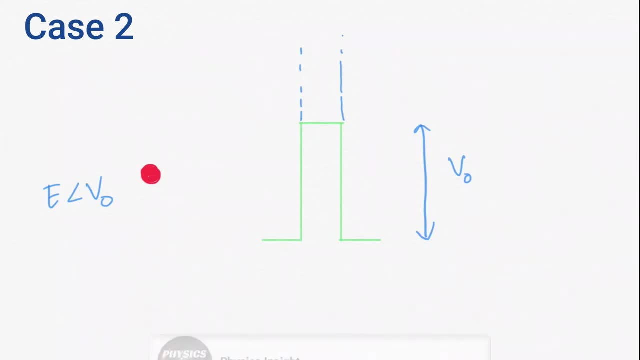 probability density function for this case. look like this. electron can be anywhere in this case. now case two: energy is less than we know. First, divide our problem in three region and name it as 1,, 2 and 3, which have different potential value. Now, on doing calculation by using schrodinger equation, we can find: 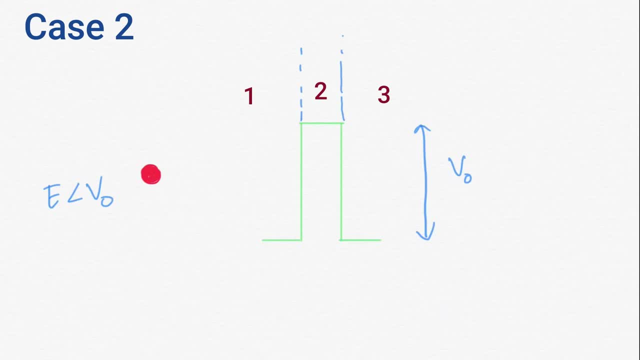 the wave function. But let's don't go to the mathematical in this video. I will make a different video on that in future. But if you are curious how we will calculate the wave function, you can see my video on finite 1D potential value for reference. It has almost. 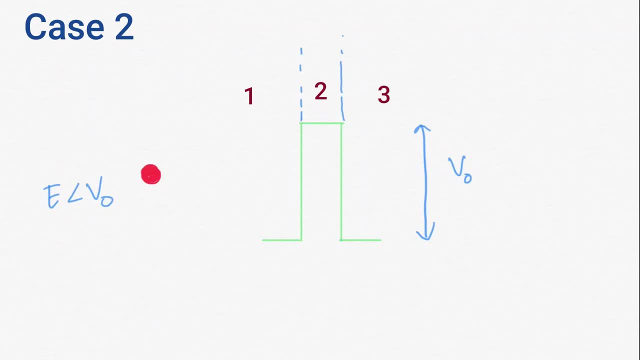 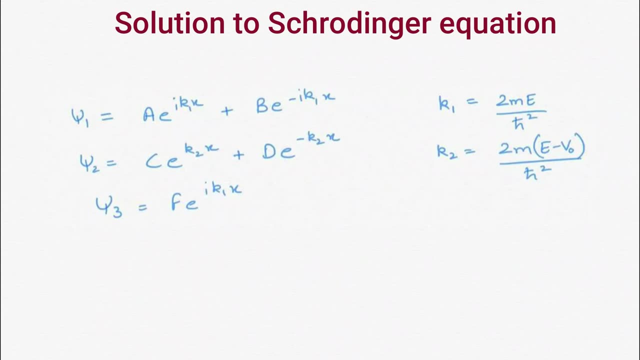 same type of calculation. So on doing calculation using schrodinger equation, we get wave function of this form in the three regions. In region 1 we have terms eik1x and e-ik1x, term which means wave is propagating along on both sides x and minus x. Term eik1x corresponds to incident. 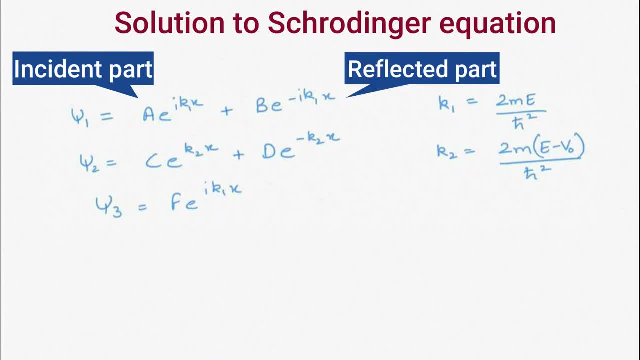 wave and term e-k1x corresponds to reflected wave and b square by a square gives the reflection coefficient. In region 3 we have wave function having term eik1x, which confirms that there are chances of finding electron there. otherwise it comes out to be zero When we plot probability density. 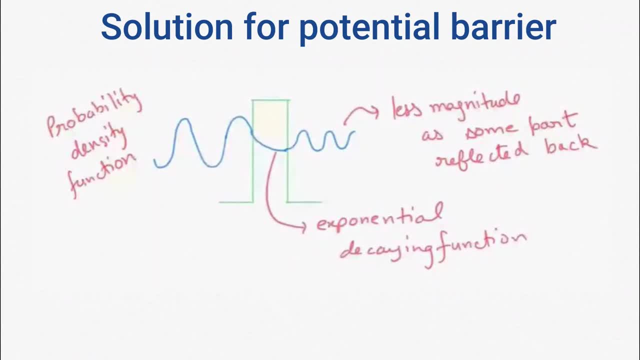 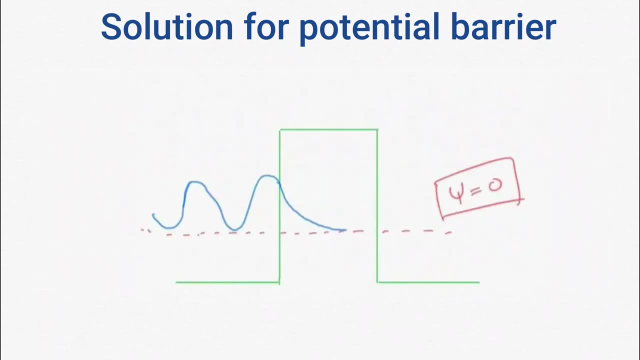 function for all three region. it comes out to be this. Now, here there is one more factor to be taken care of, as we have exponential decaying function in region 2, and if we have wider potential barrier, we may have no wave function in region 3.. 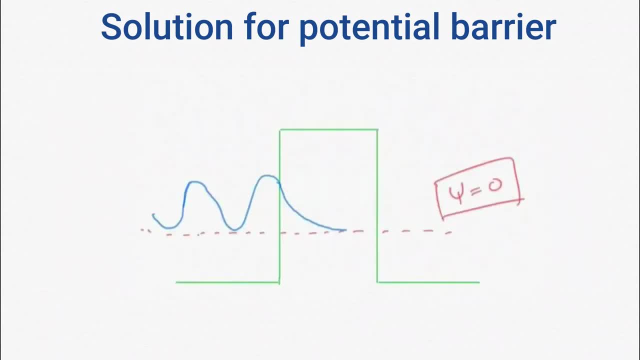 This is because the time of reflection of electron is not given by the first wave function and there is no reflection of electron in region 3 as it will die in region 2.. Means with increase in value, of width, more electron are reflected back and after a particular 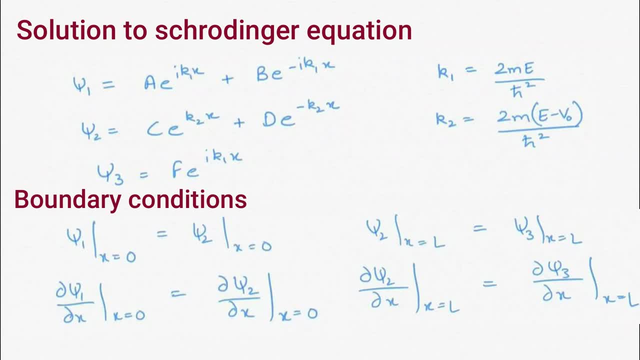 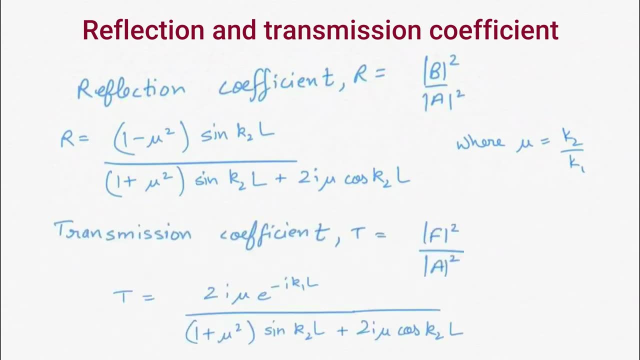 value, no electron can be there, as a result of which there is zero wave function in region. 3. Using boundary condition solution for wave function, we can find constant a, b and f, and ratio of b square by a square gives the reflection coefficient and the ratio of f square by a. 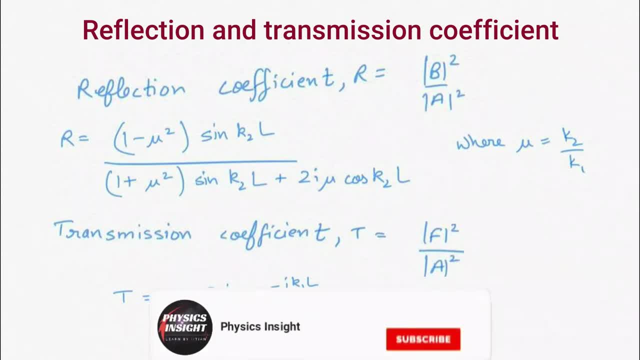 to the incident. wave b is the coefficient corresponding to the reflection wave and f is the coefficient corresponding to the transmitted wave. In expression of transmission coefficient and reflection coefficient, we see that they also depend on the width of the potential barrier. So quantum tunneling also depends upon the width of the potential barrier which is given. 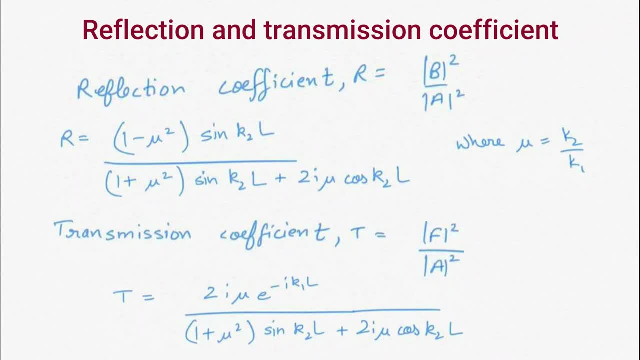 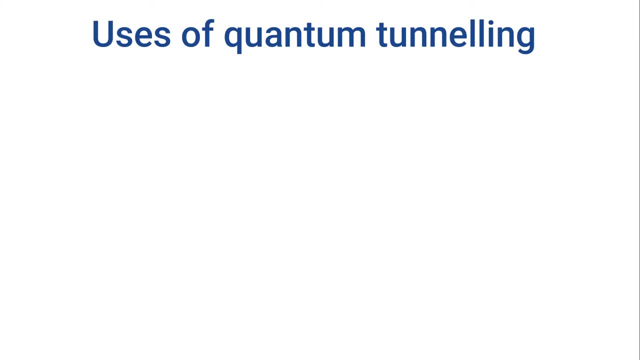 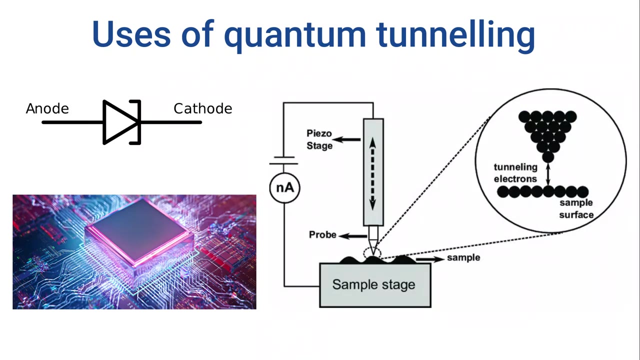 by this expression. Don't care about this expression for now. This is all mathematical. So now we have understood what is quantum tunneling. Quantum tunneling is used in tunnel drive, quantum computing and scanning tunneling microscope. So that's all for this video. 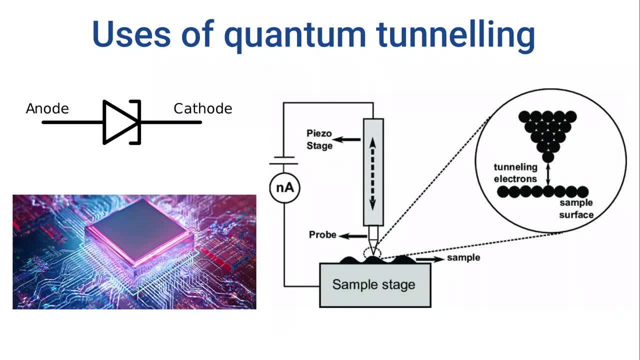 If you have watched this video till here, don't forget to subscribe to the channel. See you, guys, in the next video.